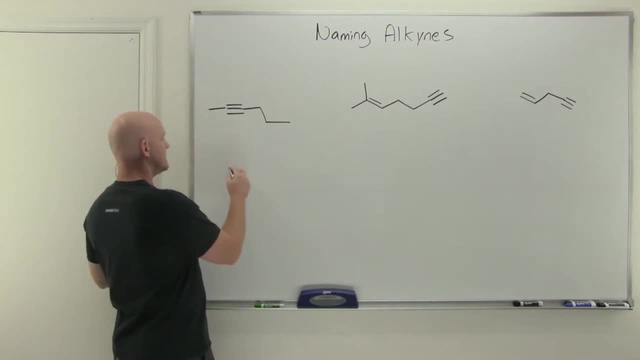 So you want to make sure you know. oftentimes we draw these things You start by drawing the triple bond First and then make sure the bonds coming off- it come off at 180 degrees, Mistake a lot of students make if they try to draw this with one, two, three, four, five, six carbons. 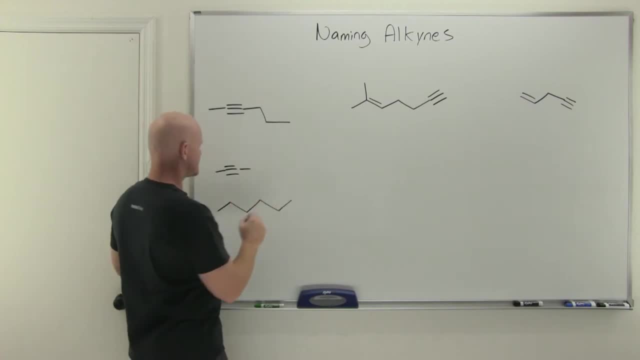 is they just do what we've done with alkanes and alkenes And they just draw six carbons and then they just shove a triple bond into the middle of it And, if you notice, that just kind of looks terrible, because it's obvious that these angles are not 180.. 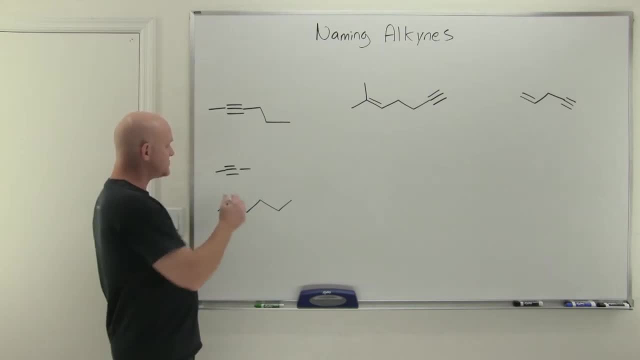 And oftentimes professors will take a half a point off on a test if you draw an alkyne like this. So by all means don't do that. A little word to the wise, but let's name this thing So: the longest continuous carbon chain. 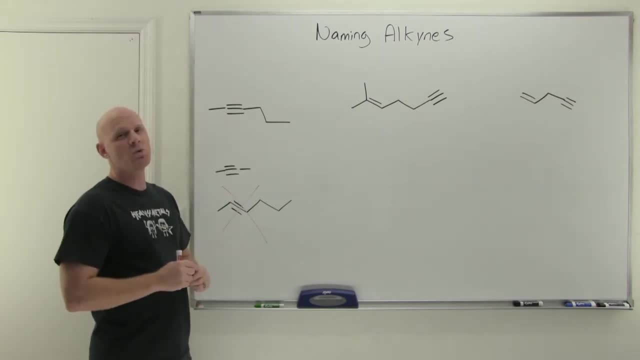 That the triple bond is a part of and number it to give the alkyne the lowest possible number. So in this case, one, two, three, four, five, six, numbering it left to right, And the alkyne is between positions two and three. 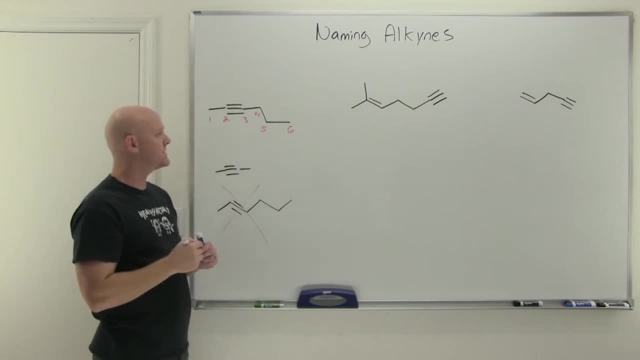 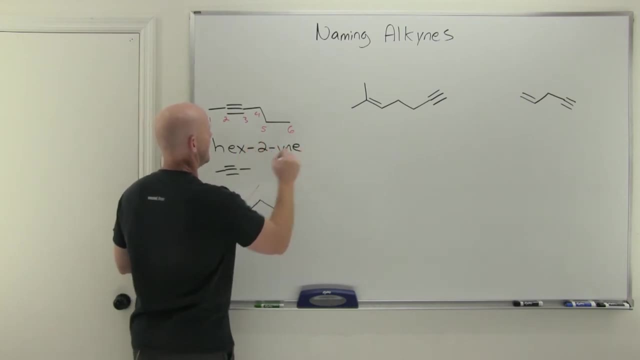 And, just like with alkenes, you give it the designation of the lower of the two numbers, And so in this case this is hex dash two, dash ein. So we use the suffix yne for alkynes. So if the alkyne is the only functional group, 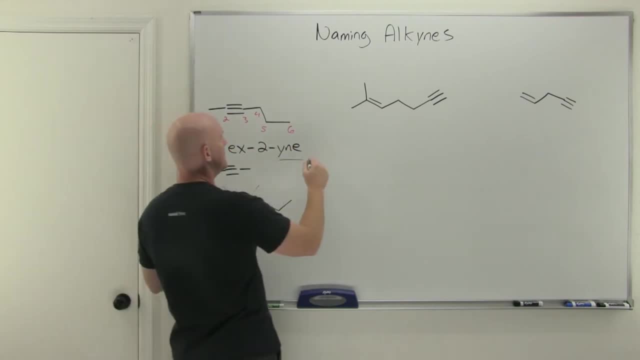 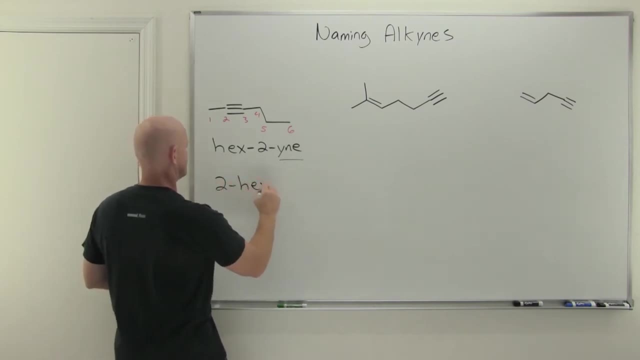 Named as part of the parent chain, Then you actually put the number out in front as well, So you could have also named this as- give myself some room here- Two hex sign as well. We'll find out later on, In fact we'll find out pretty shortly. 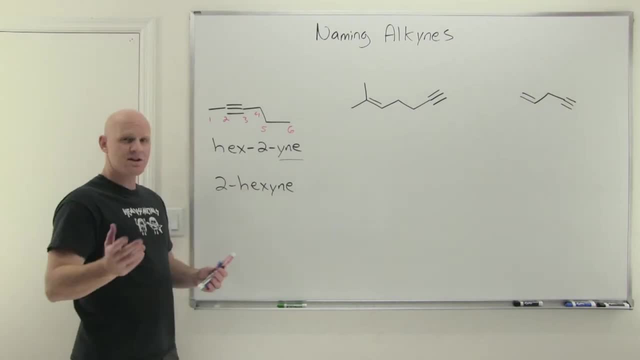 If you've got more than one functional group that is named as part of the parent chain- which is not super common, but it does happen- Then you can't put the numbers out in front of the parent chain. You're going to have to put them in the middle of the parent chain. 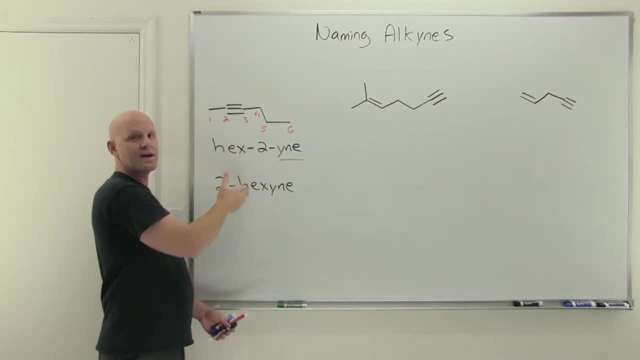 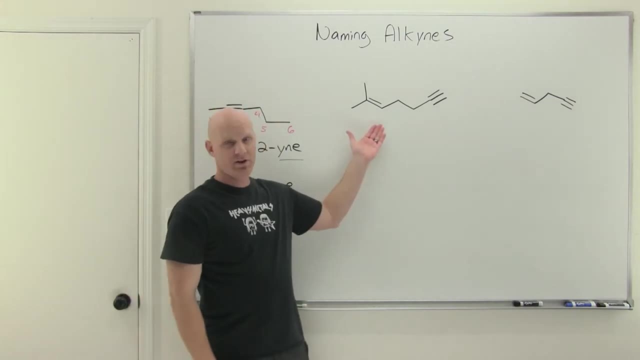 So not the worst thing to kind of get used to doing that anyways, But you're probably should recognize It either way, All right, So what if you have both an alkyne and an alkene in the same molecule? So you'll find out that we've got a whole bunch of different functional groups. 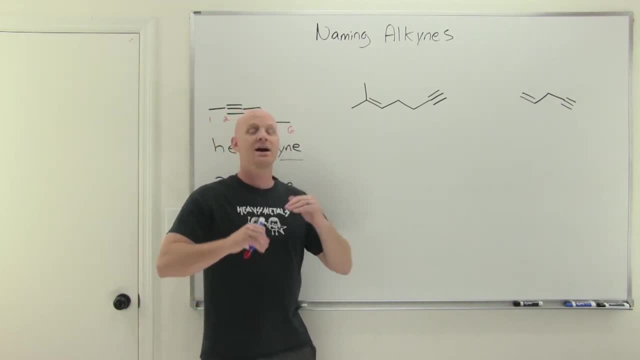 We're going to learn name over the course of these two semesters of OChem and there's a priority and you find out. based on this priority, you decide which one becomes part of the parent chain And then oftentimes you'll find out. the other one gets named as part of the uh substituents out in front of the parent chain, but with alkenes and alkynes they can both show up in the parent chain at the same time. 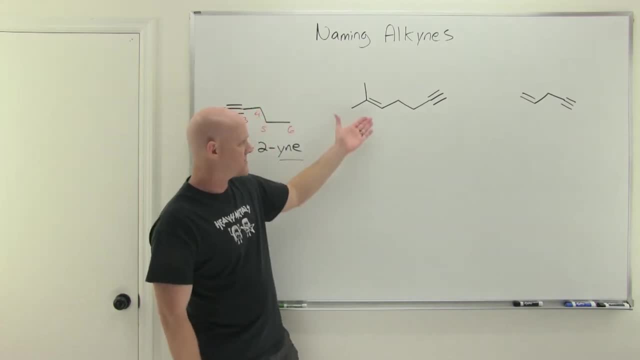 And you call it an ein. So you get both the ein and the ein here. So, and it turns out though that which one gets, the priority is not set. It actually determines is determined numerically first. If the alkene can get the lower number, the alkene gets the priority. 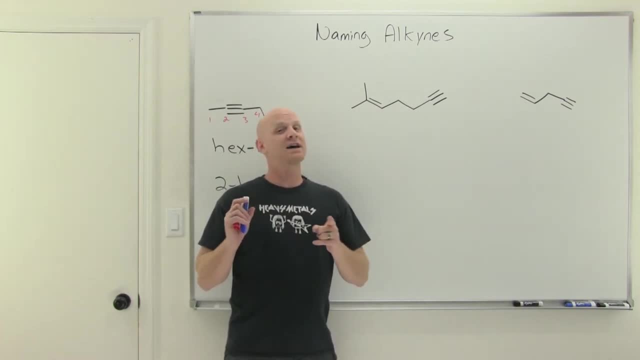 If the alkyne can get the lower number, then the alkyne gets the priority, And if it's a tie, we'll find out like it'll be on this last one. We'll find out that the alkene gets the priority on the tiebreaker. 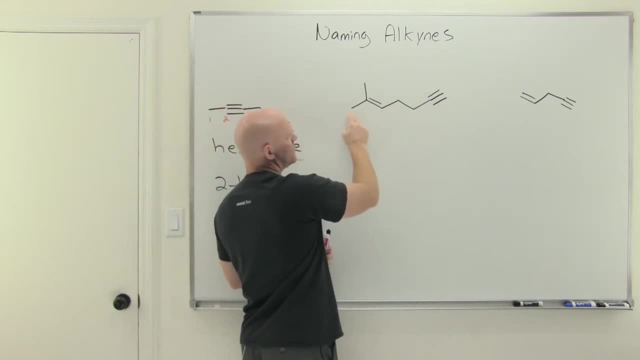 All right. So in this case, longest chain that contains both the alkene and the alkyne is one, two, three, four, five, six, seven carbons. So this is going to be some form of hex-ein-i. 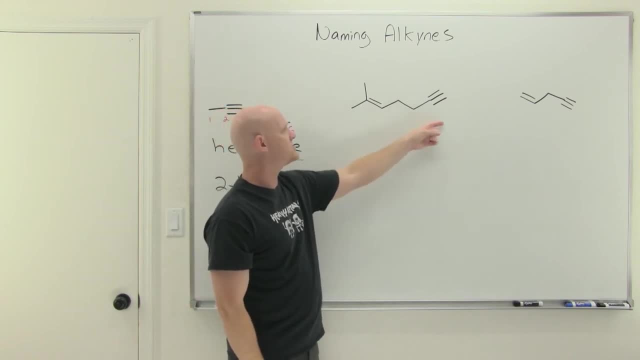 So hex-ein-i, And in this case, if I number it left to right the chain, I'll see the alkene at carbon two. If I start from the right-hand side, though, I'll see the alkyne at carbon one. 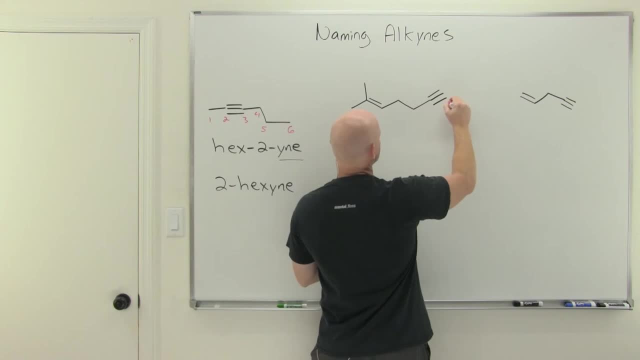 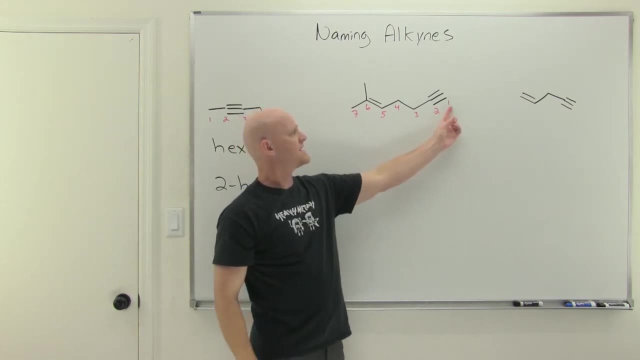 That's lower numerically and that's going to be the preference here. So whichever one you can get a lower number is going to get the priority. All right. So we see the alkyne is at position one and the alkene is at position five. 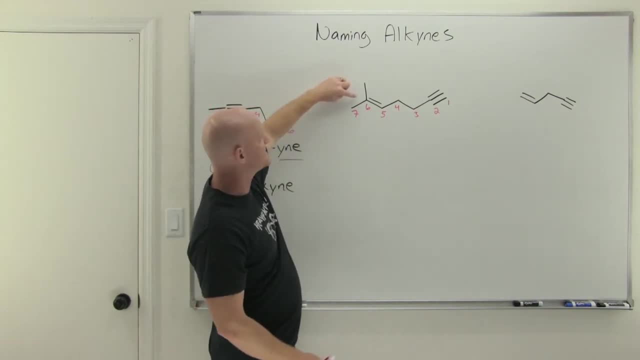 And don't forget that anytime you name an alkene you should check for E and Z. But in this case the sp2 carbon on the left-hand side here is bonded to two identical methyl groups. And once again, if either side is bonded to two identical groups, no E and Z, no cis and trans isomers possible. 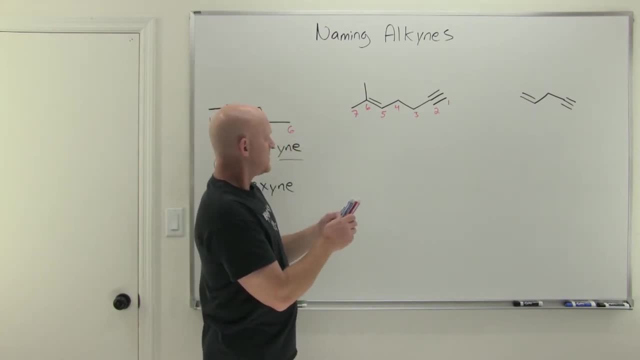 It only exists in one way, So we don't have to worry about that in this case. So, but in this case, we also have this substituent right here And we'll name the substituents first, just like normal, And we'll start off with six methyl. 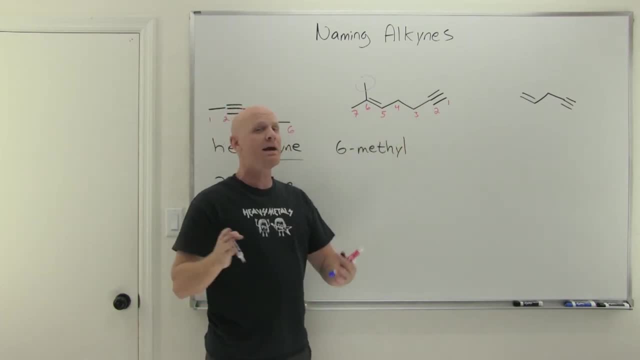 So, and in this case, because the e and the ein are going to both appear in the parent name, the numbers have to go in the middle of the parent name. So six methyl, and then hept for seven, And then ein comes before ein. 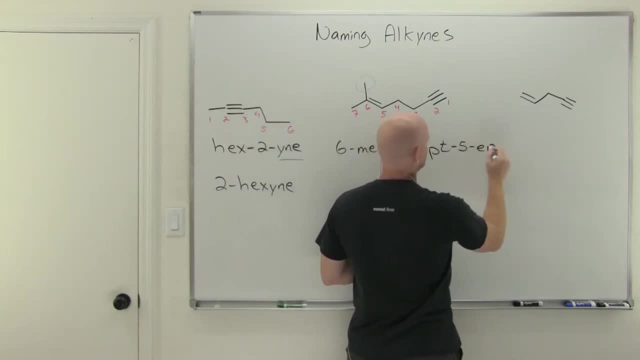 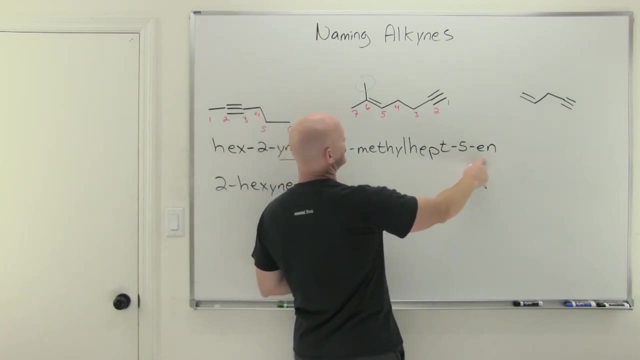 And so it's at position five. So hept-5-ein, And we'll drop the e, since we're about to say ein. We don't want vowel-vowel combinations in the parent chain here, So hept-5-ein-1-ein. 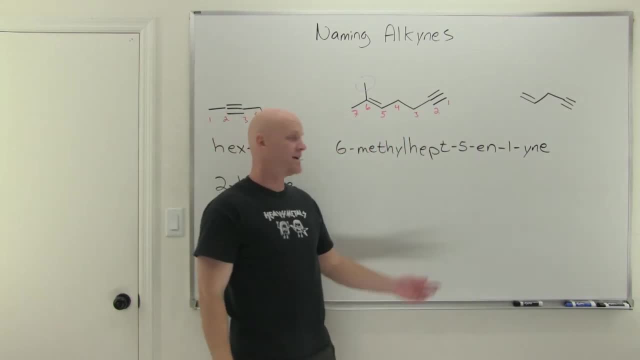 Cool, And there's our lovely name: six methyl hept-5-ein-1-ein. And again, because there's two major functions showing up in the parent chain, the numbers have to go in the middle of the parent chain. 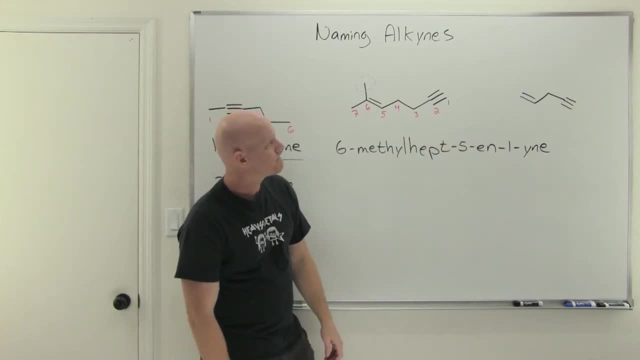 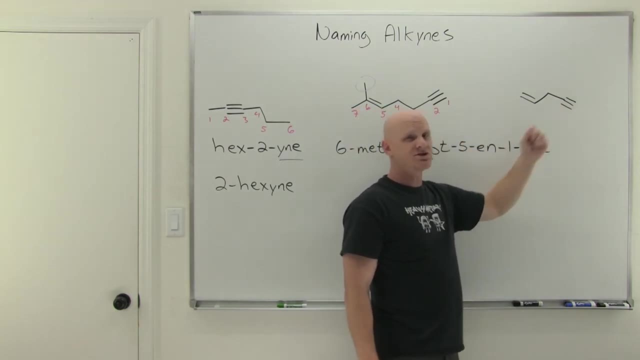 You couldn't pull them out in front of the hept, It would not work. All right, So finally, this last one. So if I number this left to right, so the alkene would be at position one. If I go right to left, the alkyne would be at position one. 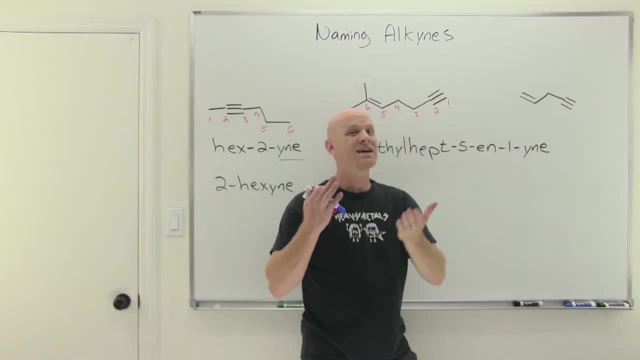 And that's when there's a numerical tie. And in this case, if there's a numerical tie, the alkene gets the priority, not the alkyne. Just the way they decided it. So we'll number this left to right as a result. 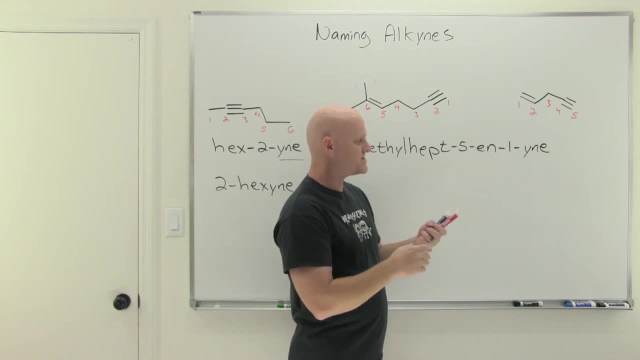 All right, And so in this case there are no substituents. Everything's contained as part of the parent chain, And it's five carbons, So we'll start with pent. So, and in this case again, ene first. 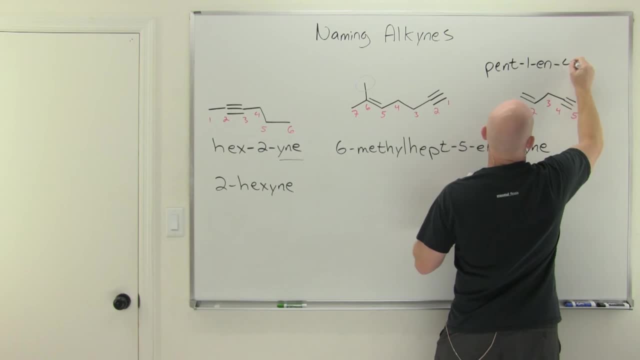 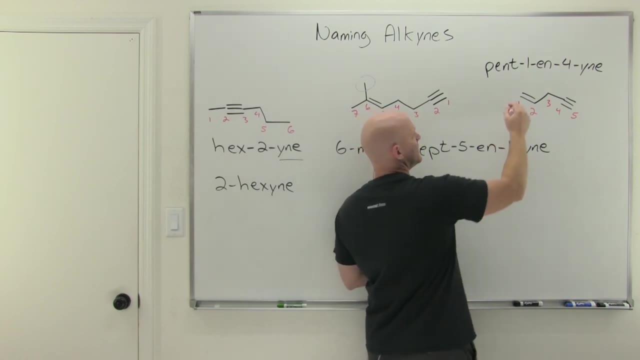 So pent-1-ene-4-ine. So, and in this case again, anytime you name an alkene you should check for E and Z, But once again they weren't drawn in, But the left-hand sp2 carbon of the alkene was bonded to two identical hydrogens. 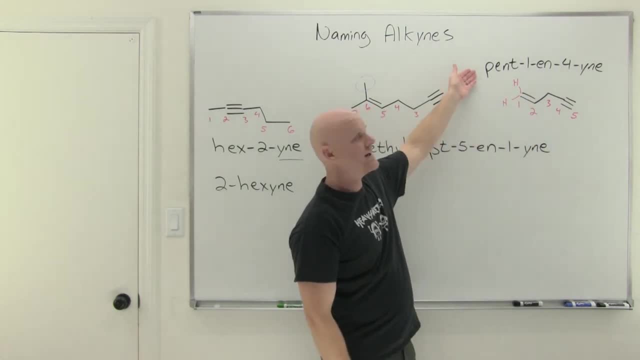 So there is no such thing as E and Z to worry about, And that is our complete name for this last one, Pent-1-ene-4-ine. If you have found this lesson helpful, would you consider giving me a like and a share? 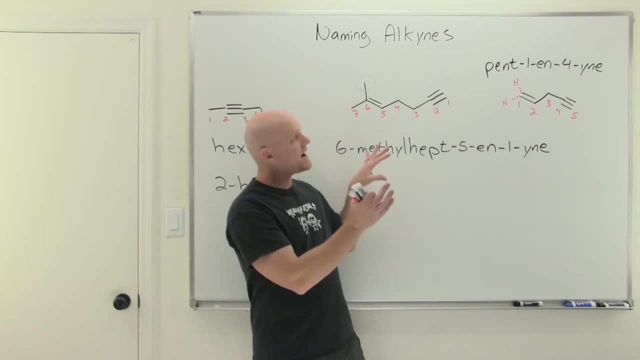 A couple of the best things you could do to help support the channel, And if you're looking for practice problems or the 168-page set of study guides that goes with my premium course, check it out on chadsprepcom. 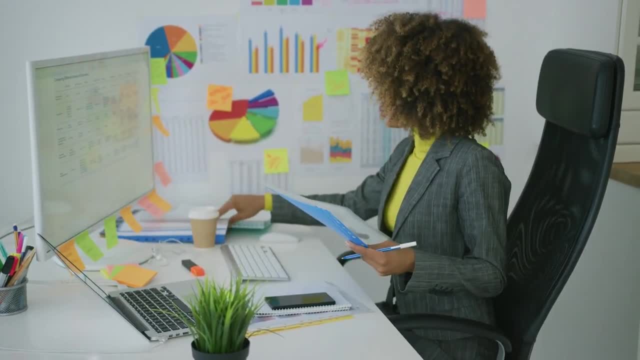 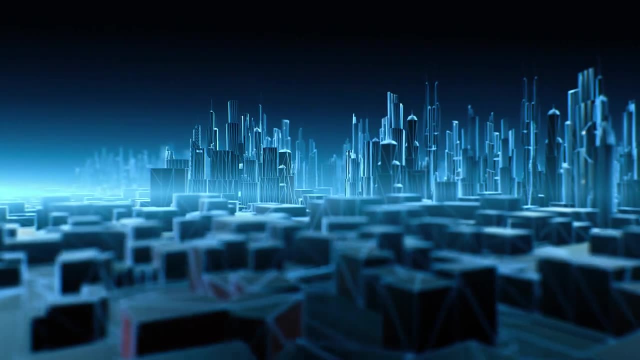 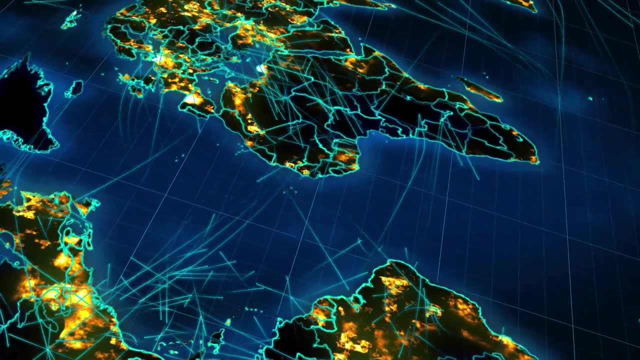 Operation research analysts build and apply models to help stakeholders and management make intelligent decisions. In this video, we're going to help you answer the question: should you become an operations research analyst in 2021?? We're going to go over the latest salaries, job market statistics and the latest trends coming up.